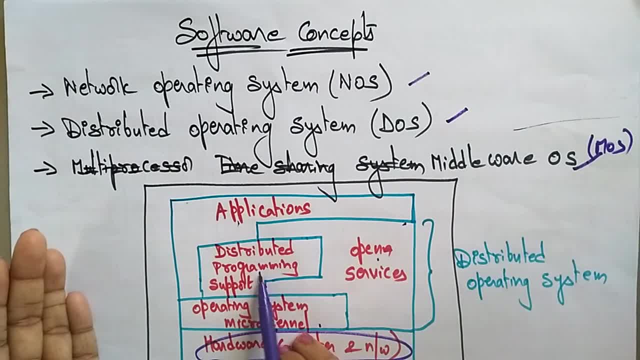 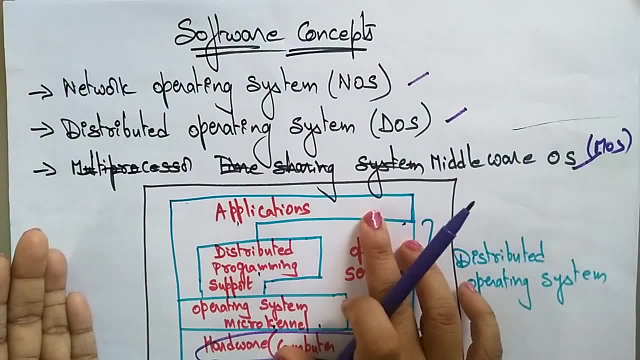 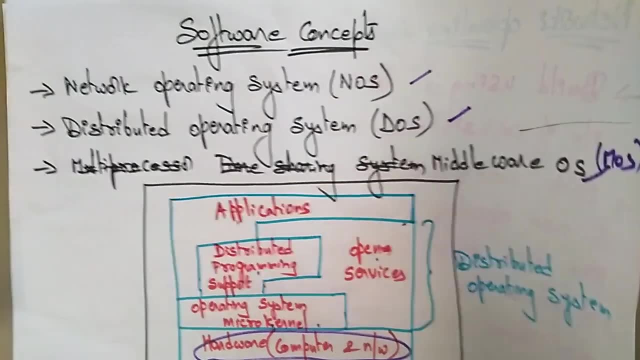 completely. this structure means the open services, distributed programming, support and the operating system. microkernel comes under the distributed operating system. Okay, and this here the applications is. it's somewhat it's a middleware operating system and the hardware is a computer and network operating system. So let me explain you one by one. first, what is a network operating system? 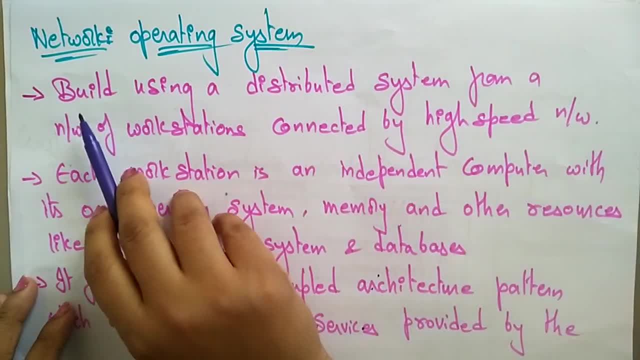 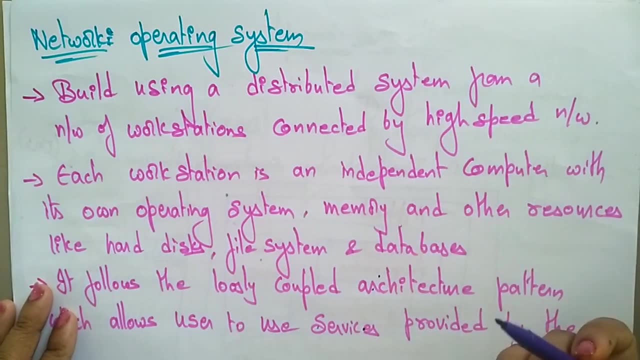 A network operating system here, the it build using a distributed system from a network of workstations connected by high speed network. So if you take a distributed system, a distributed systems- all are connected- means some workstations. workstations means nothing but the nodes, The nodes. 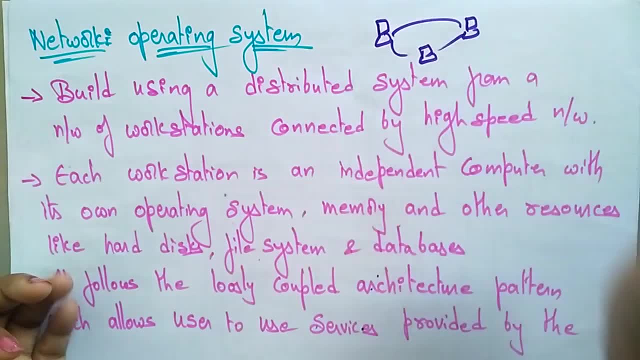 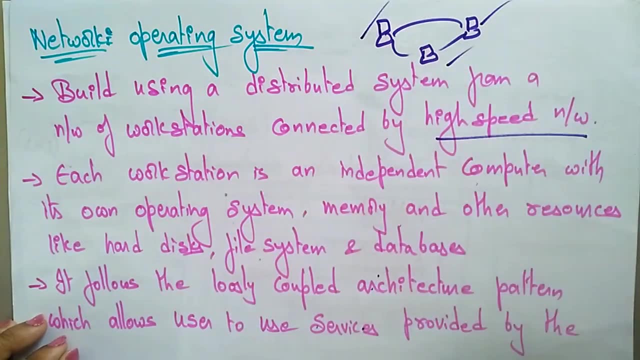 are all connected. So you have the workstation and the structured system All connected, all connected with a high network, high speed network. Each workstation is an independent computer. So whatever the workstation that you are taken, that is an independent computer. It is independent. 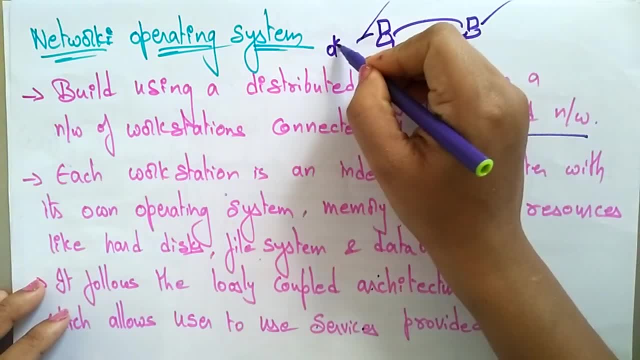 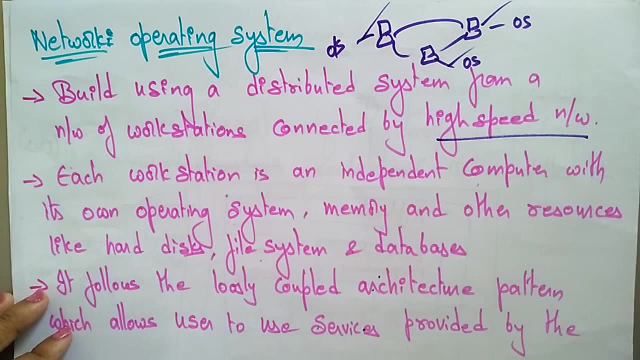 So everyday system is an independent with it's own operating System. So each workstation has the operating system. their own operating system will be present memory and other resources like hard device, file system, database, smoother main. So we said a neural network is a homesuite data structure and a high speed users is also possible to connect the high speed data. So every workstation from country to another place is a whole network delivered all connected along high speed network. Each workstation is an independent computer. VOWS is connected offline. 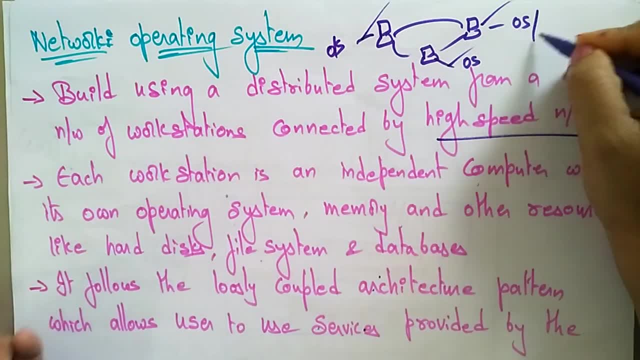 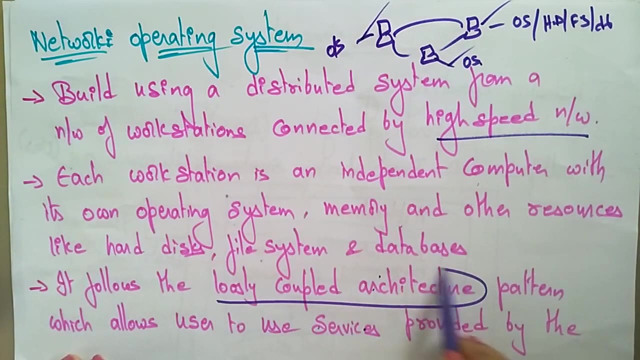 system is independent of the other system. so each system is having the operating system, hard disk and file systems and even the databases. each system is having these components. it follows the loosely coupled architecture. the one thing that you have to remember- that the network operating system, nos, is a loosely coupled architecture. it's not tightly. tightly means 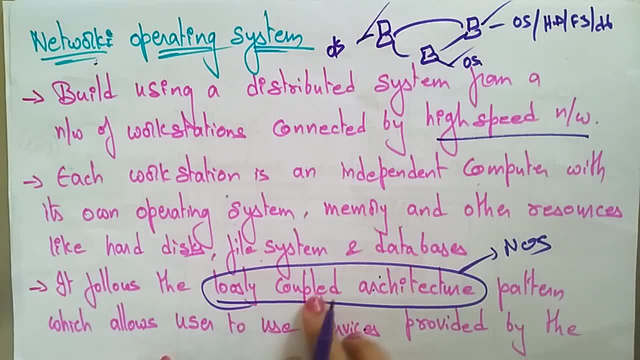 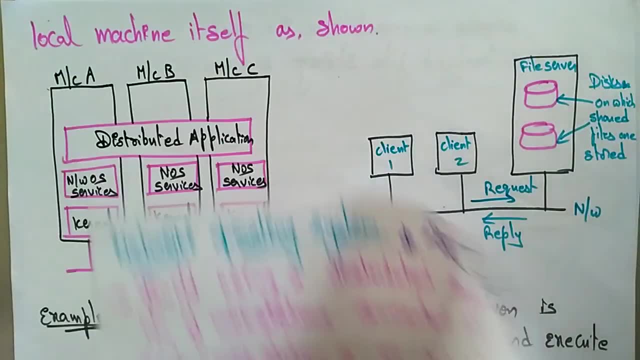 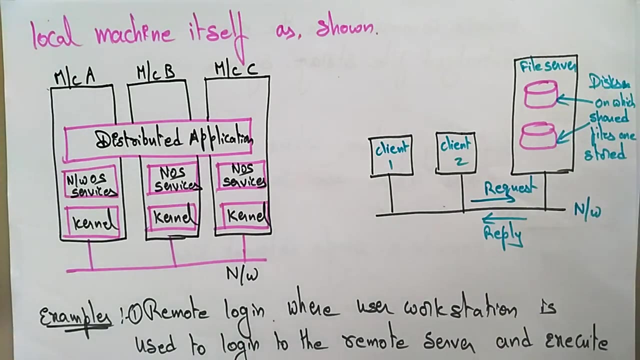 it's a shared memory. loosely means distributed system. it's a loosely coupled architecture pattern which allows user to use services provided by the local machines itself. so why, uh, network operating system is a loosely coupled architecture? because the pattern, whatever you are going to be arranged, the systems that follows the user to use services provided by the local machines itself. so just see. 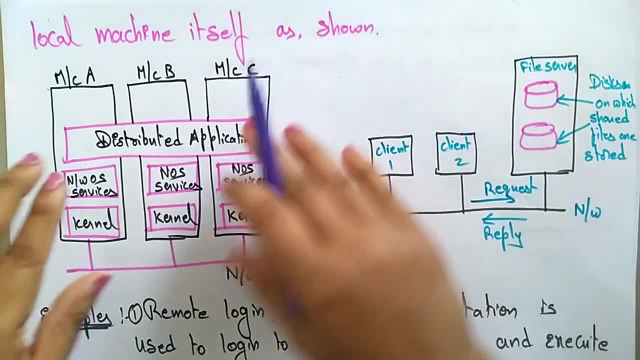 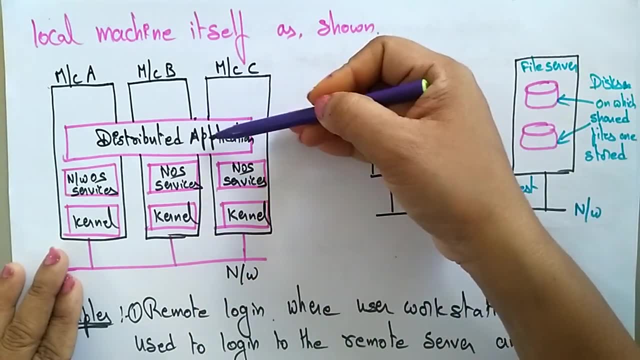 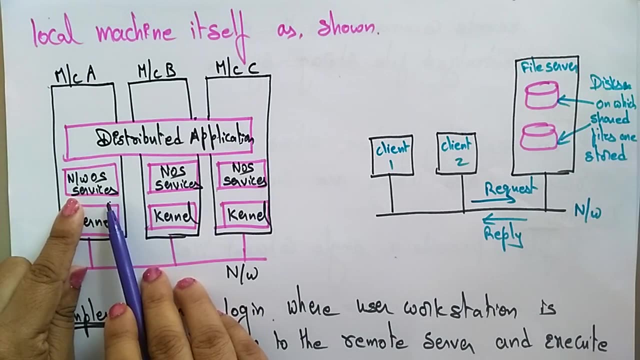 here. this is the diagram here, the machine a, machine b, machine c, three machines. let's take three machines. each system is independent to other system. so here the system is having the distributed applications and each system housing nos, that is a network operating system service. each machine is having their own network operating. 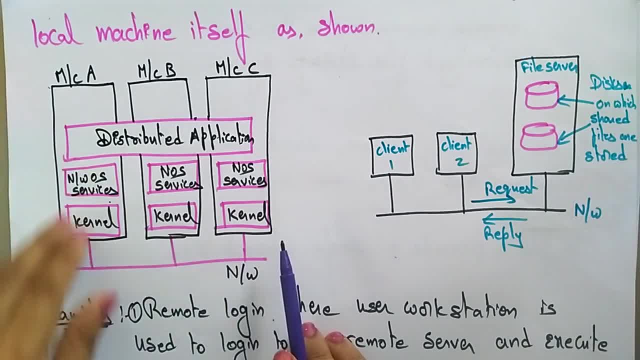 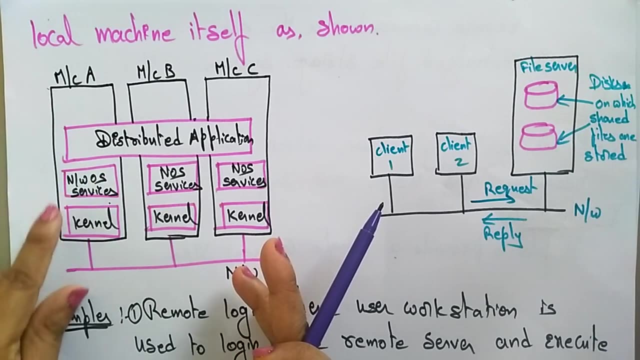 system services and a kernel will be connected, and all the systems is connected with a network. so, by seeing this diagram, what do you understand here? uh, each workstation, this is a workstation. each workstation is an independent computer with its own operating system. there is a network operating system. 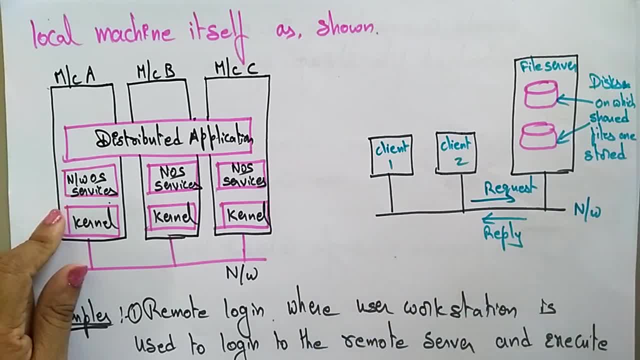 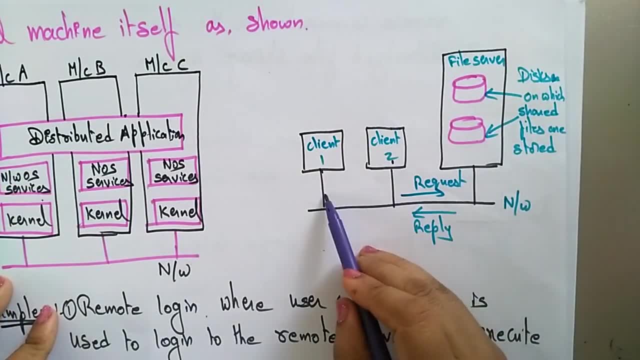 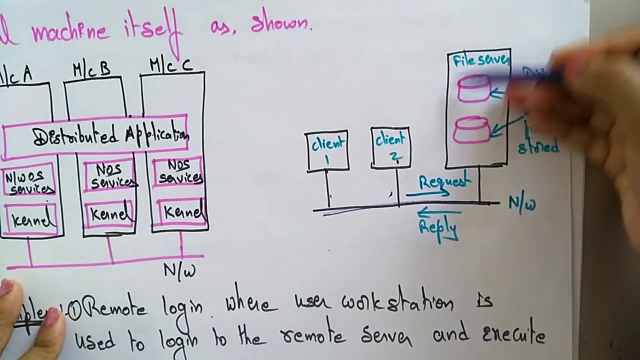 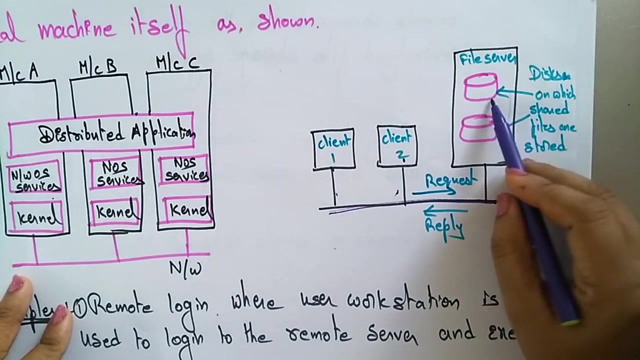 and the memory and other resources like hard disk, file system and database. okay, so see, see, here is a client one and a client two. these client one, client two are connected over a network. okay, and uses a server, the file server. so these two clients are using file server. the file server is having the database means it's a disk on which 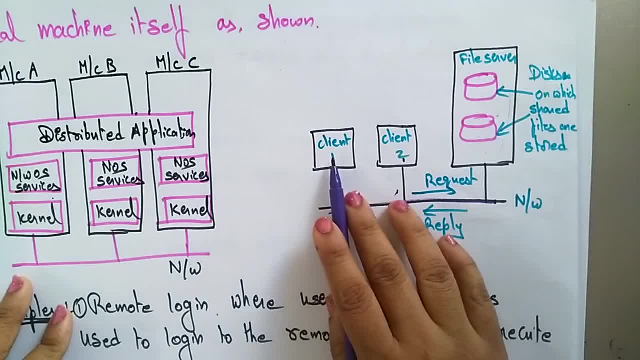 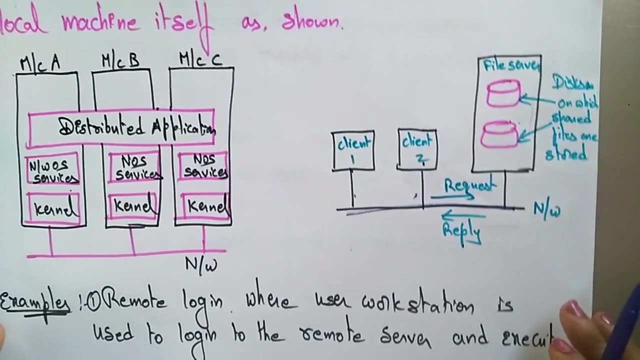 shared files are stored. so whenever the client- uh, client, if client one requires, it requests the file server. and if a client wants the files, it requests the file server. so the file server is replying. so now let's see some examples of this network operating system. the examples are the: 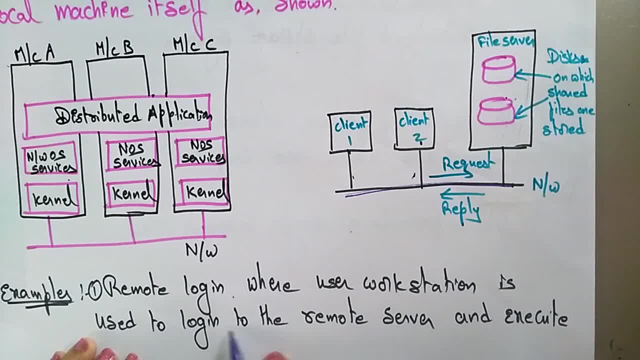 remote login where user workstation is used to login to remote server and execute. so here you can say: this is a user one and the user two. the user want to access this file. how he is going to access the file? he has some remote login means with the username and the password. so is user to? 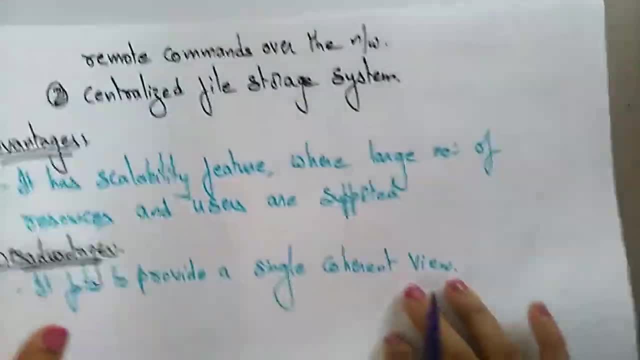 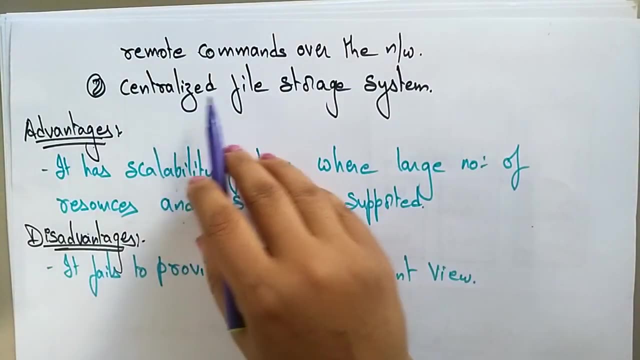 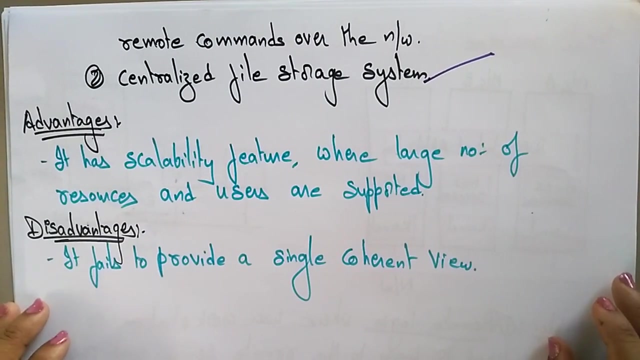 login to remote server and execute the operation. the remote commands over the network and the second example- here it's, the network operating system- is a central, central, centralized file storage system. Now let's see what are the advantages and disadvantages in network operating system. The advantages are: it has a scalability feature where large number of resources and users 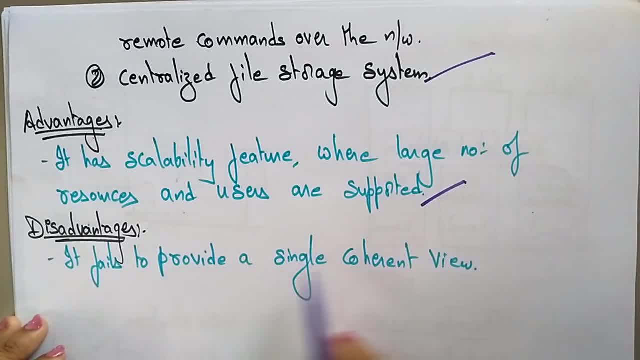 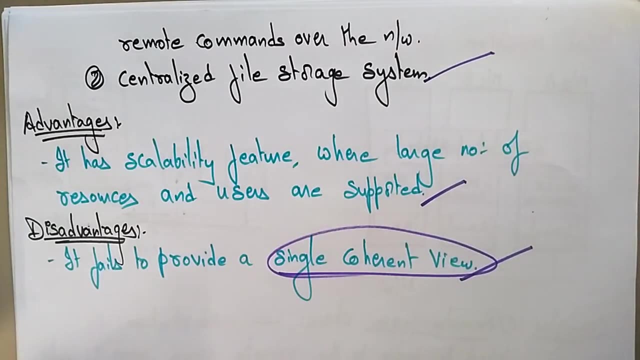 are supported. and disadvantages: it fails to provide a single, coherent view. So the main disadvantage in using this network operating system is it's going to fail. it fails to provide a single, coherent view. So this is about the network operating system. Thank you.